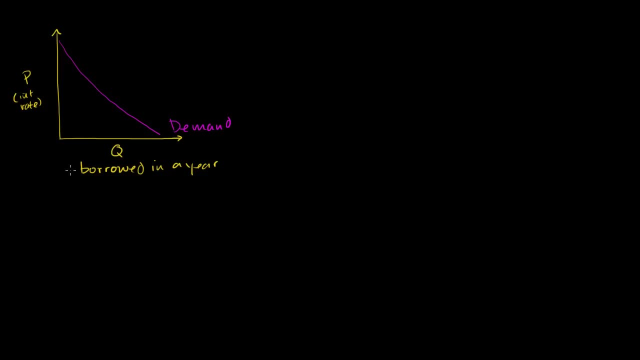 And the supply curve, and once again this is the exact same logic we use with the demand supply curve for any good or service. for money might look like this: Those first few dollars. someone has a very low opportunity cost of lending it out, So they're willing to lend it out at a very 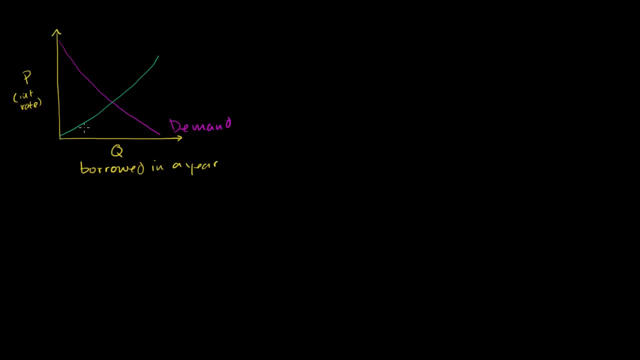 low interest rate, And then every incremental dollar after that there's higher opportunity costs, And so people will lend it out at a higher and higher rate, And then you have a market equilibrium interest rate. And so let me copy and paste this, And then we can think about: 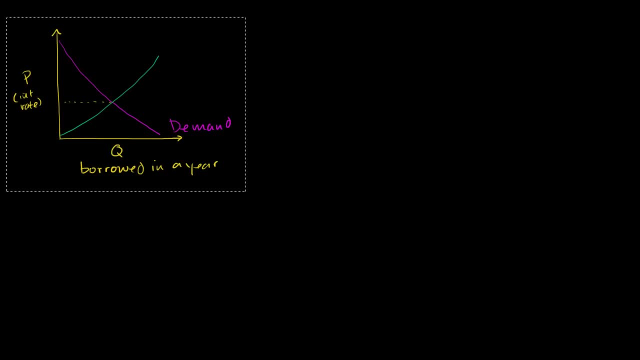 what happens in different scenarios, So copy and paste. So now we have two scenarios that we can work on, And then let me just do one more Three scenarios. Now let's think of a couple. Let's say that the central bank of our country- and in the United States that would be the Federal Reserve- 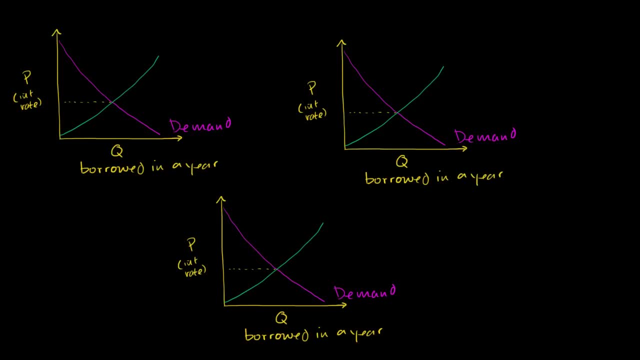 the central bank prints more money and then decides to lend out that money, And that actually does not happen. And in the previous video I talked about the central bank printing money and then dropping it from helicopters. That is not how money is actually distributed. It is distributed. 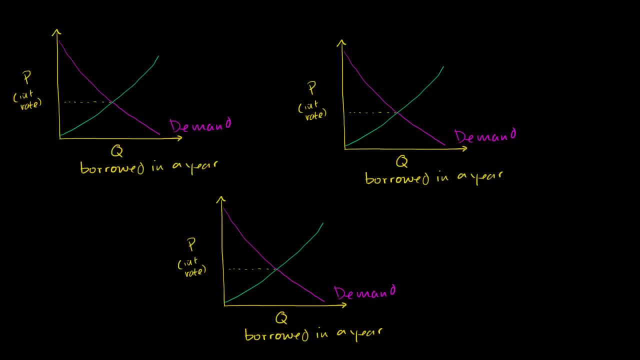 when central banks print money, the way that it enters into circulation in most countries is that the central bank then goes and essentially lends that money, the way it's done in the US Fed. For the most part, they go out and buy government securities, which is essentially lending money. 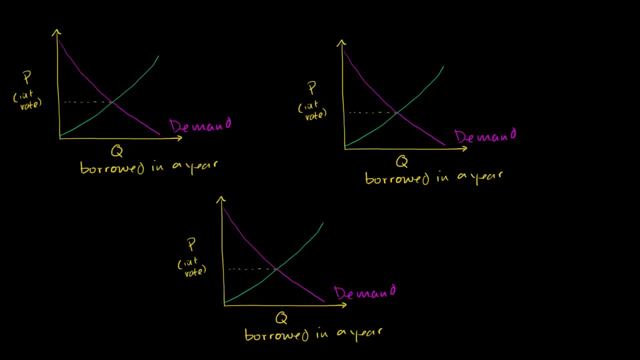 to the federal government, And they do that because that's considered to be the safest investment. But the central bank then goes out and buys government securities, which is essentially lending money, And so if some more money? so if this is our original supply curve, if this is our original, 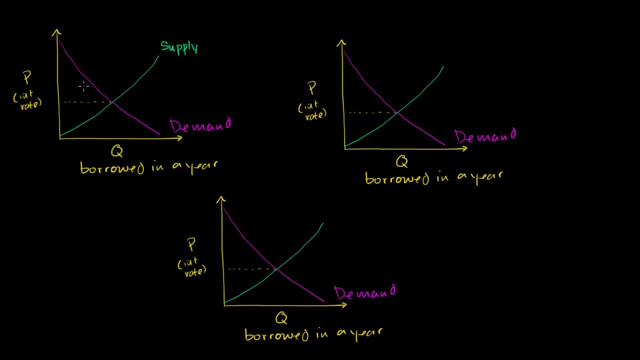 supply curve. but now your federal, your central bank, is printing more money and lending it out. what is going to happen over here? Well, your supply curve is going to shift to the right. At any given at any given price, at any given interest rate, you're going to have a larger. 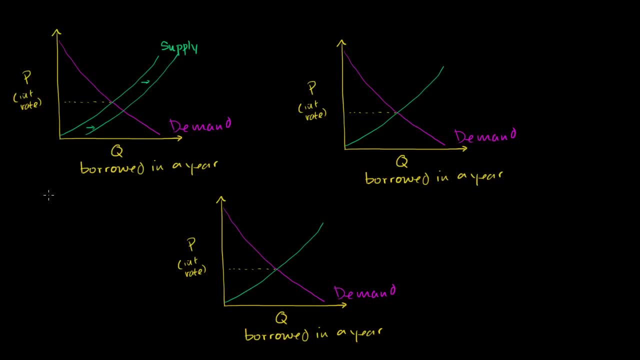 quantity of money being available. So it might look something like it might. your new supply curve is going to look something like that And, assuming that's the only change that happens, you see its effect: Your new equilibrium price of money, the rent on money or the interest rate on. 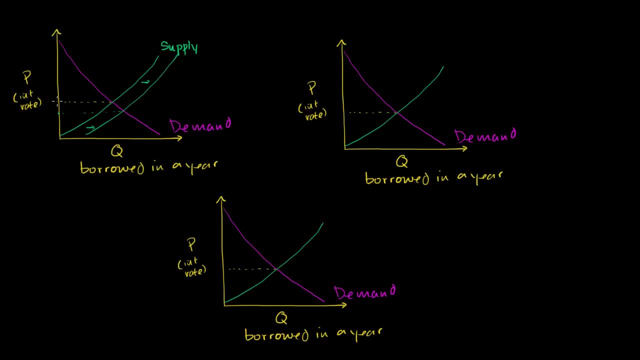 money is now lower, And that's why, when the, when the federal reserve says I want to lower interest rates, they do so by printing money, and they print that money and they lend it out in the market And that essentially has the effect of lowering interest rates. Now let's think about another. 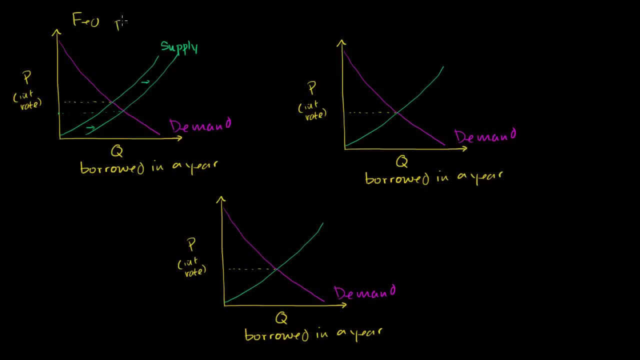 situation. Let's say so. this is, this is the Fed prints, prints and lends and lends money, lends money And they're lending the money by buying government bonds. When you buy a government bond, you're essentially lending that money to the federal government, And I've I've done other videos on that. where we go into 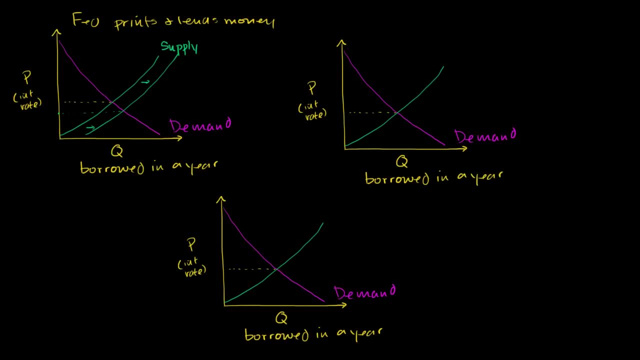 a little bit more detail on that. Now let's think of another situation. Let's think about consumer consumer savings. consumer savings go down. So one interesting thing about savings: savings in investment are two opposite sides of the same coin. So when you save money, so money you literally. 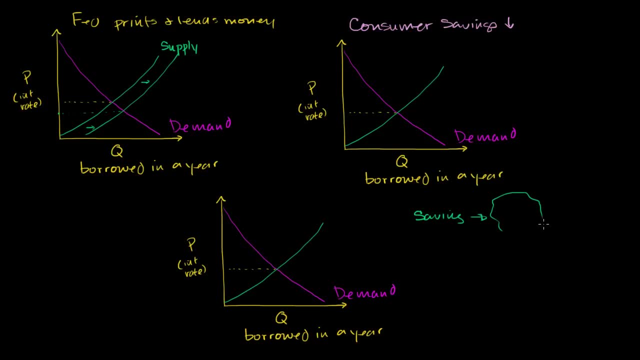 put it into a bank so that you have the whole financial system right over here. So this is the financial system, financial system. that money is, then goes out and it is lent to other people And then, for the most part, hopefully, that money, when it's lent, is used to invest in some way. 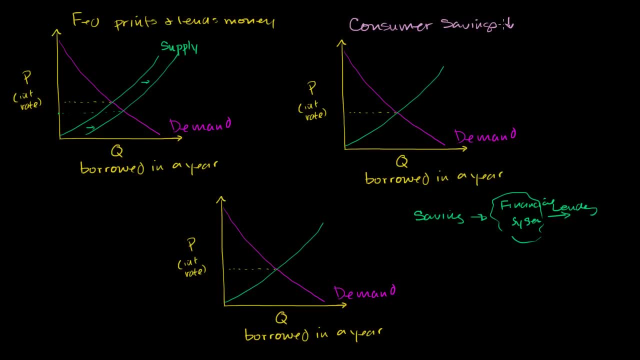 So this is lending. So if consumer savings goes down, that means that the supply of money will be shifted to the left At any given price or any given interest rate. there will be less money available. So in this situation, our supply curve. 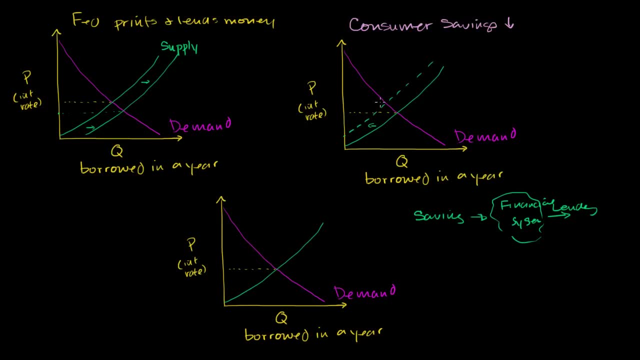 is shifting to is shifting to the left, And just that would increase interest rates. And then you could even make an argument that if consumer savings is going down, consumers are borrowing, are going to borrow less as well, And you could argue that maybe demand would go up as well. And 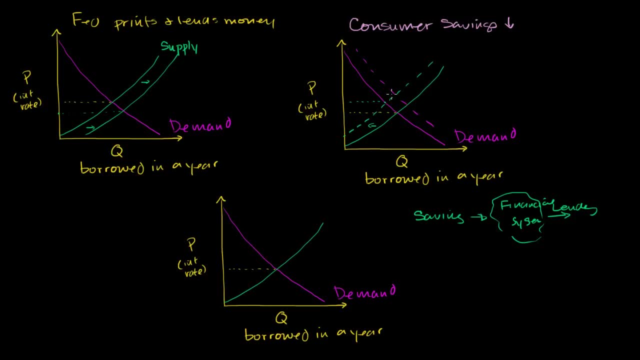 so your, your demand could go up and that would make that would make the interest rate go up. And then you could make an argument that if consumer savings are going down, consumers are borrowing equilibrium interest rate even even higher. Now let's do another scenario. 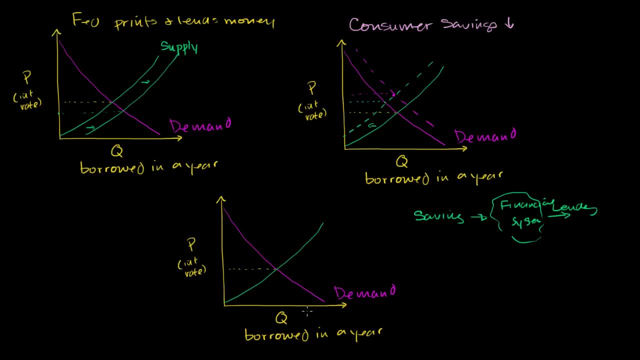 Let's say that the federal government, in an effort to- let's say that they, for whatever reason, they're trying to finance a war or some type of public works project and they don't want to raise taxes, so the government decides to borrow a lot more money.